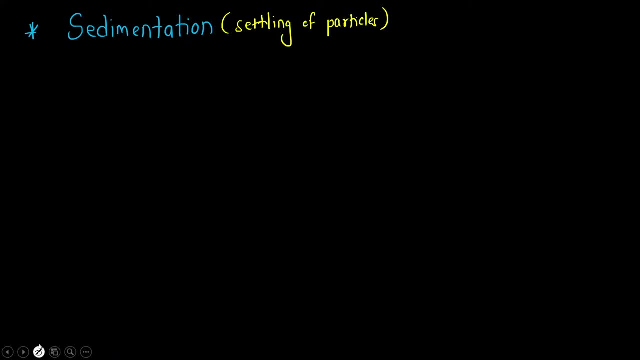 So somehow we have to settle these particles. Now, this settling of particles- we can say sedimentation. it is divided into four types. Okay, So there are four types of sedimentation, Four types of settling, Four types of settling. 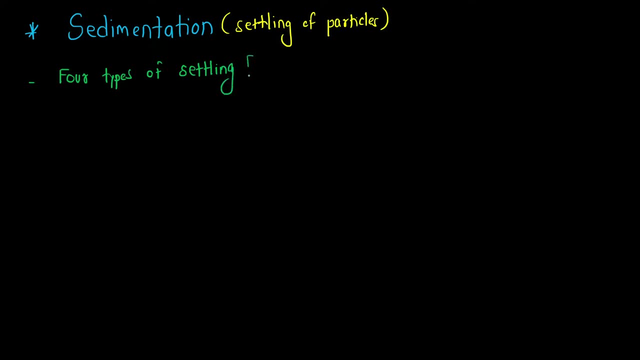 Now this four types are based on interaction of particles. Okay, So they are based on the interactions of particles. so what are the four types? so the first one that is called as type 1 settling: type 1 settling. so we have discussed this. 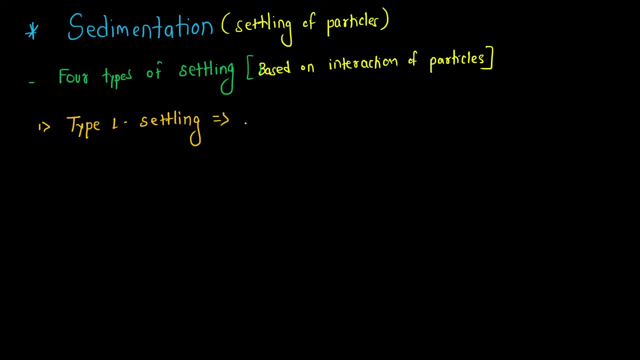 in the plane sedimentation. so type 1 settling is also called as discrete settling. it is also called as discrete settling, that is, settling of discrete particles. now what is the meaning of discrete particles? the particles will do not change their shape and size. okay, no change in shape or size. so we found, we find this in: 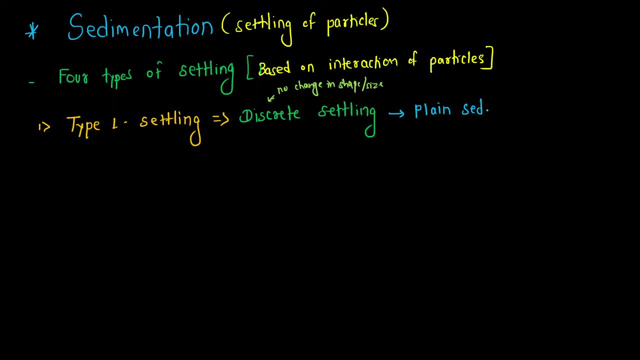 the plane sedimentation tank: plane sedimentation tank. okay, now the second one is called as type 2 settling, type 2 settling. this is called as flocculent settling, flocculent settling, flocculent settling. where do we find this flocculent settling? we find this in: 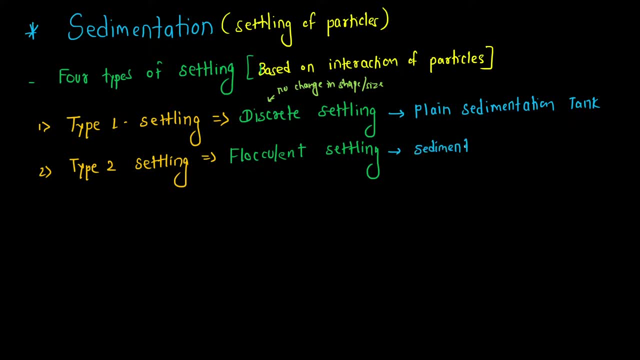 sedimentation added with coagulation. sedimentation added with coagulation, coagulation. okay, now what is the meaning of this? flock or flocculant? see these discrete particles, these discrete particles, these are the alone particles which are settling. okay, so in the plane sedimentation tank, the particles which 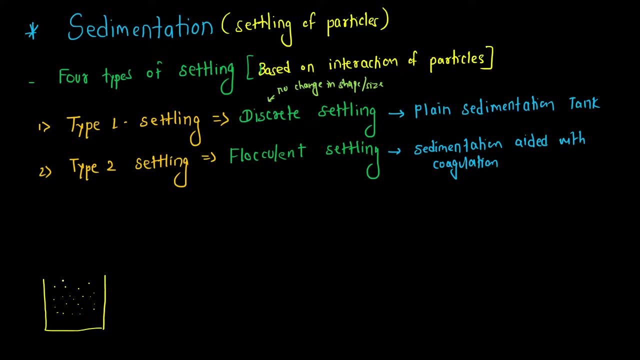 get removed. that is, in the type 1 settling, the particles which get removed are nothing but the suspended solids. okay, now, smaller than suspended solids, we have colloidal solids and dissolved solids. so to remove these, this particle size is very less. okay, the size of particles is very, very less. so what we 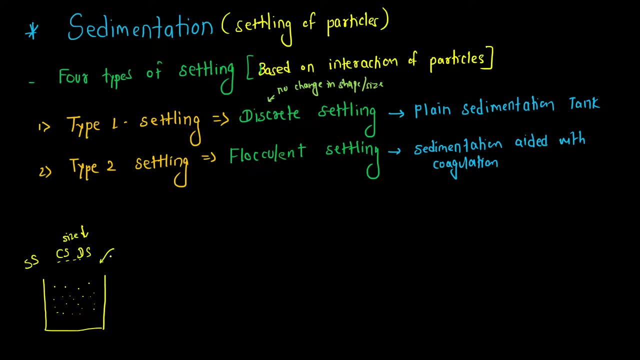 do is we add, we add some chemicals in the liquid so that these small, small particles they stick to each other. okay, what we are doing, see, whatever the larger particles are there, that is, suspended particles. these particles have certain weight so they settle directly. or we can say easily at: 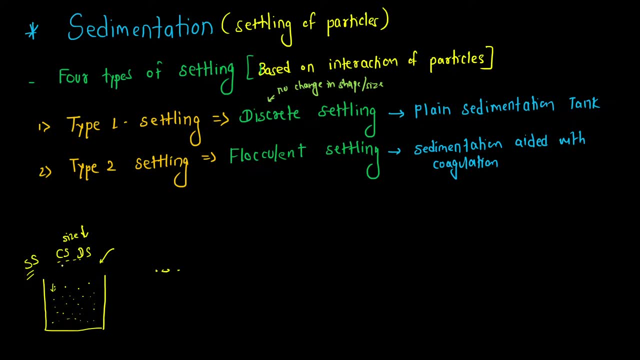 the bottom and they can be removed. but these colloidal solids and dissolved solids, their size is very, very less and they will take a lot of time to settle down, or even maybe they will not settle down. also they will. they will keep on being in suspension as their weight is very, very less. now what we will do is 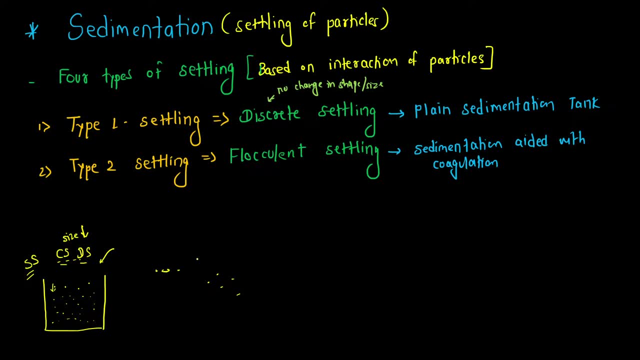 let's say this: these are some colloidal solids. they are very, very small, so they are less low. now what we will do is, let's say these: these are some colloidal solids, so we will add some chemical here. okay, so we'll add some chemical here, due. 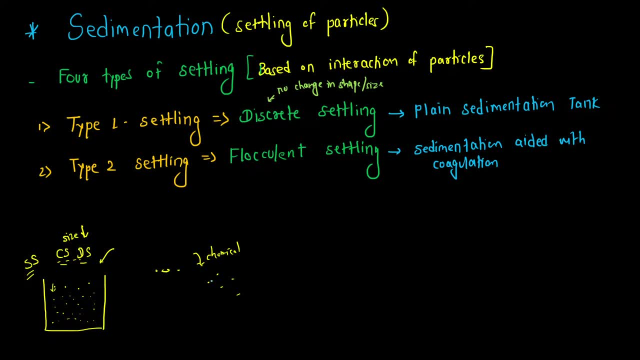 to this chemical. what will happen? there will be inter particle bridging of this particle. that means these particles will stick to each other. now you can see, the five individual particles have become a one, a big particle. so this big particle, which you can say due to the addition, 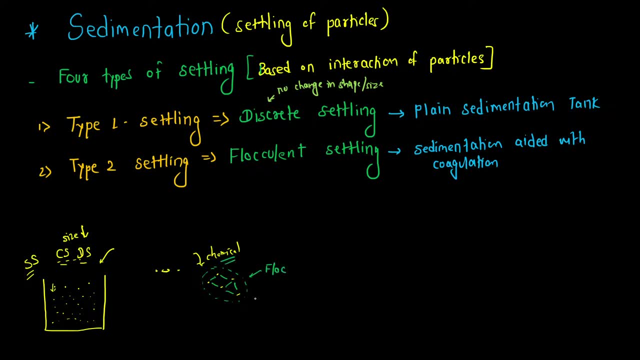 of the chemical is called as a flock. okay, this is called as a flock. now, as this particle is bigger, its weight is also higher. okay, so its weight is more. so this settles easily. so this is what we call it as flocculant settling and the chemical which is used. the chemical which is used for 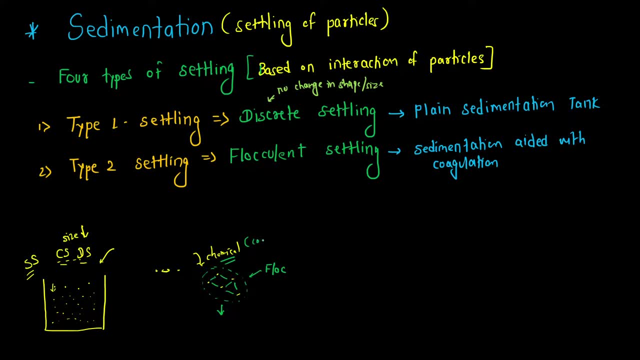 inter particle bridging of these particles is called as coagulant. coagulant, okay, and the whole process, this whole process is called as coagulation. i hope it is clear now. so these big particles, or these flocs which are settling down, this settling, this type of settling, is called as type 2 settling. 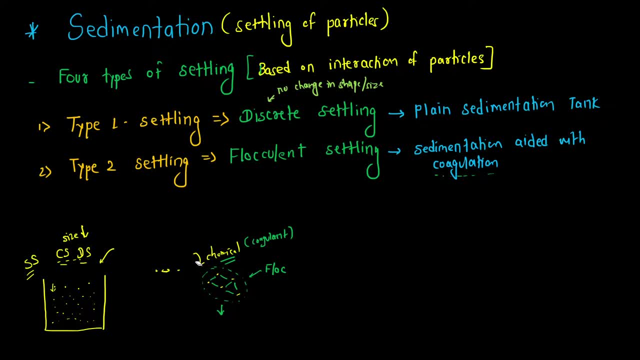 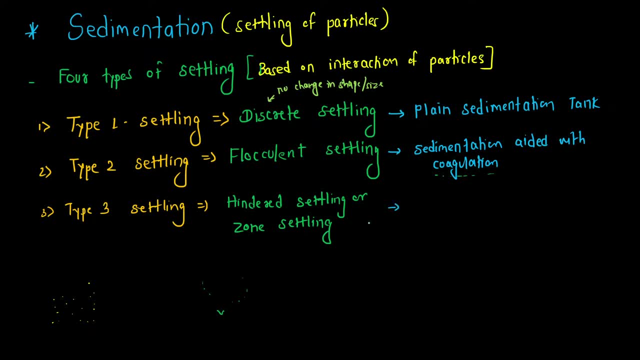 now the next type of settling, that is, type 3 settling, and it is found in sedimentation added with coagulation. now, where do we find this? now, where do we find this? so we find this in secondary sedimentation tank of activated sludge process. 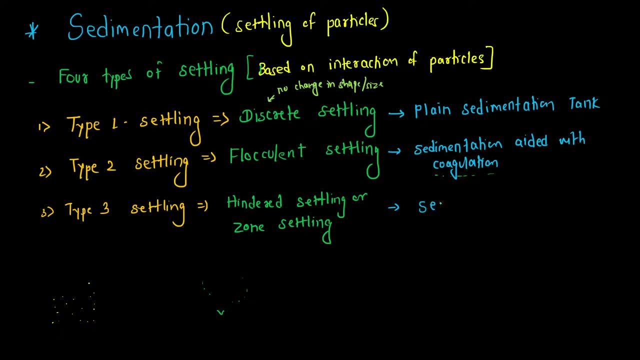 so we find this in. so we find this in of activated, of active sludge process. okay, now the last one, that is, type 4. so type 4 settling, this type of settling is called as compression settling, compression settling and we find this compression settling in. 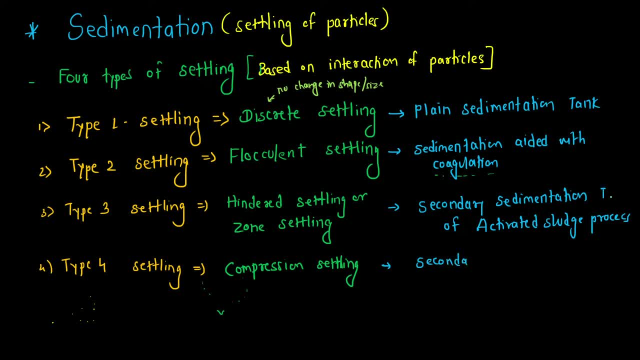 secondary sedimentation tank. secondary sedimentation tank of trickling filter. ok, now, these are the most important types of settling, or we can say, in sedimentation. so this part is very, very important computer exam point of view. so you should remember this. which type of settling occurs? 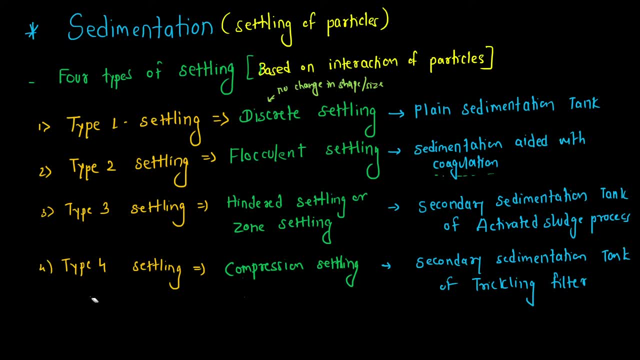 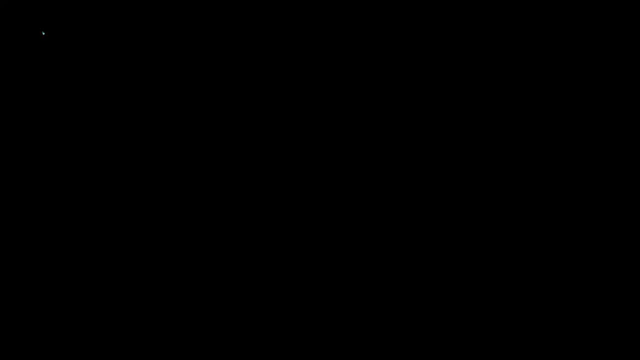 and what is the name of the settling and in which unit it occurs. ok now, so one more point we will discuss here. that is called as primary clarifier, so give the heading primary clarifier. so this primary clarifier is similar to. it is similar to primary sedimentation tank. 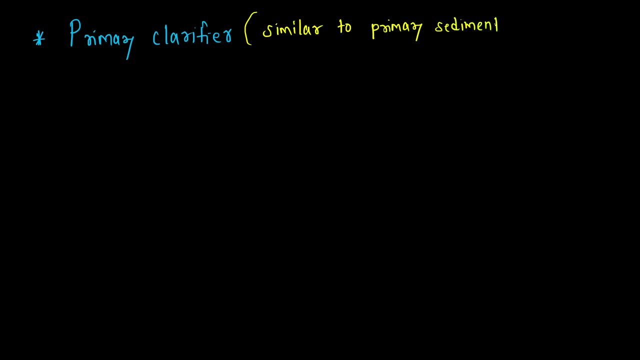 or we can say plain sedimentation tank, plain sedimentation tank. so the functions are also same. so it is nearly same. only so the primary clarifier settles down the organic solids which are present in waste water. so primary clarifier settles down settlable organic solids. 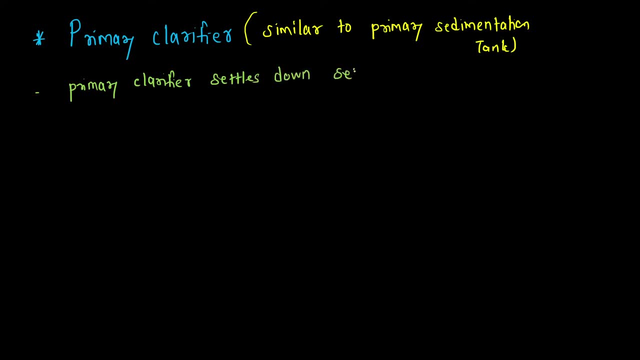 which are present in waste water, so primary clarifier settles down. so it is similar to that slowly these organic solids which are present, so they settle with the passage of time due to the settling of particles so same as the plain sedimentation tank. so the particles which are getting 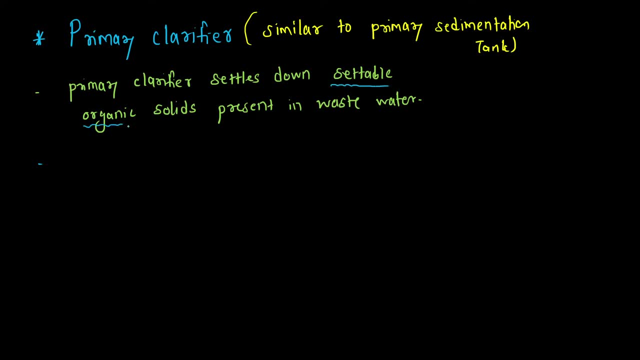 settled here are settlable organic solids. now primary clarifier: primary clarifier removes, so it removes 60 to 70 percent, 60 to 70 percent of organic solids and 20 to 30 percent of BOD. okay, so this is the percentage BOD which is. 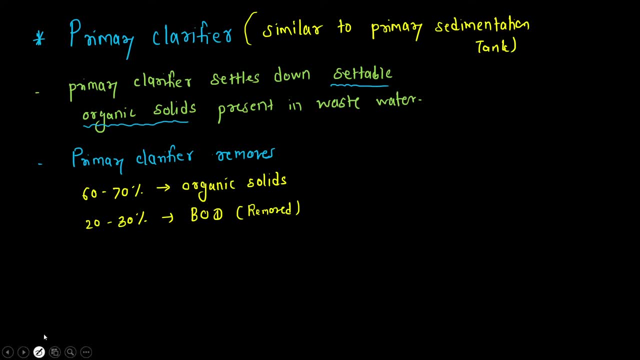 removed. now which type of settling is seen in the primary sedimentation tank, or we can say primary clarifier, so type 3 settling. type 3 settling is found in primary clarifier, so type 3 settling is called as. what is the name of the type 3 settling, hindered settling or zone. 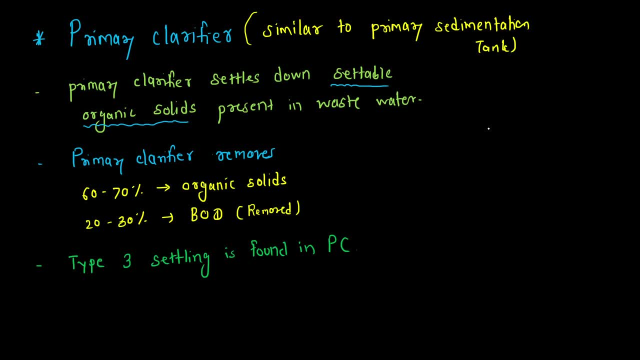 settling, hindered settling or it's own settling. so let's say this is a primary clarifier. now, in this primary Clarifier, the sewage is present立 of the Type 3 Settling is called as. What Is The Name of Type 3 Settling인�q. 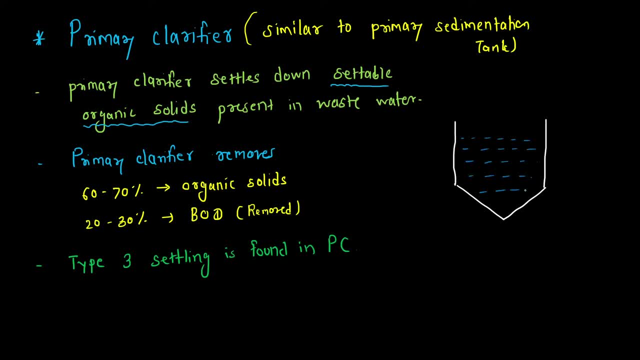 anicful Settling Design, incomprehensible public discourse hoje. I don't know the title of Title of the Type 3 Settling are presented in order. in View Point 5, Type 3 Settling Is foundwegen Z censored and it is allowed to settle now. as usual, there are certain organic impurities which are present. 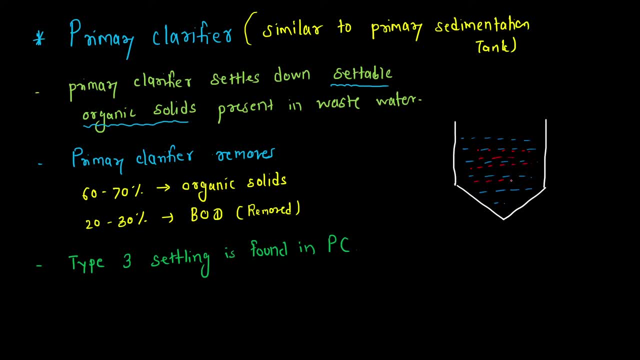 now the concentration of these impurities is higher as compared to the discrete partling settling. okay. so, due to the high concentration, what happens is that there is inter particle, inter particle interaction of particles, or you can say there is hindrance of the particles, so there is hindrance of one particle to another, see, as the concentration is higher. so when 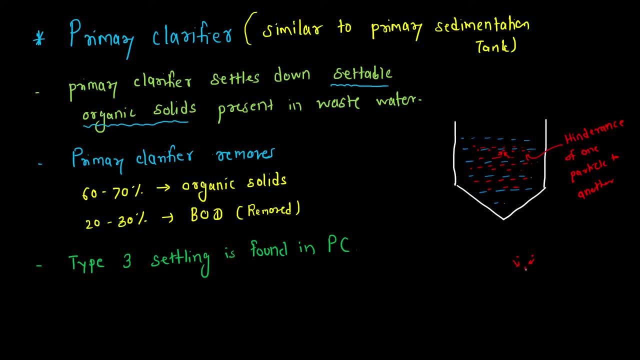 the particle settles its, it collides with each other and there is certain hindrance to the settling of the particles. so this hindrance is thereby given the name as hindered settling. okay, so, due to the hindrance of particles. so these are the important points about primary clarifier. 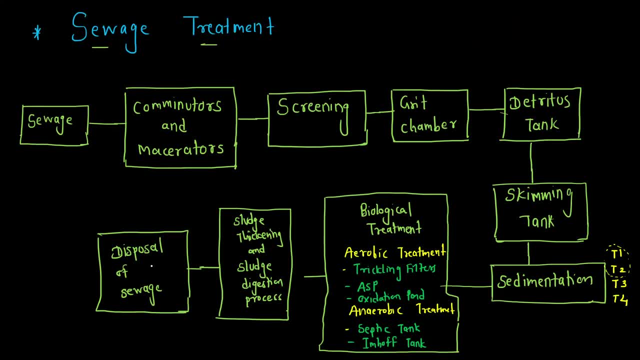 now in our diagram which we are studying right now about this sewage treatment plant. so before the biological treatment starts, there is one sedimentation unit which is given. okay, so before the biological treatment starts, there is one unit which is given here, and this is called as primary clarifier. okay, now, after the biological treatment is done, there is: 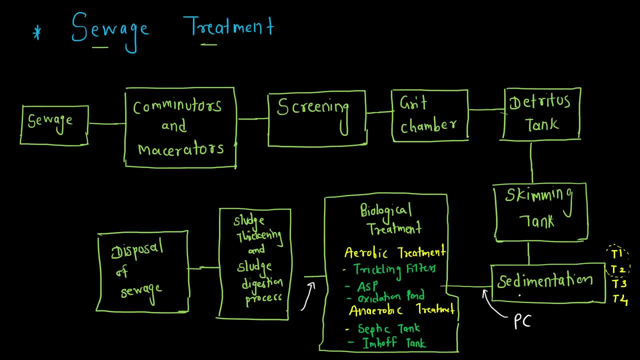 one unit which is given here. there is one sedimentation tank, which is given here, and that unit follows the same sedimentation principle and this is called as secondary sedimentation tank. okay, or you can call it as primary sedimentation tank and this is the secondary sedimentation. 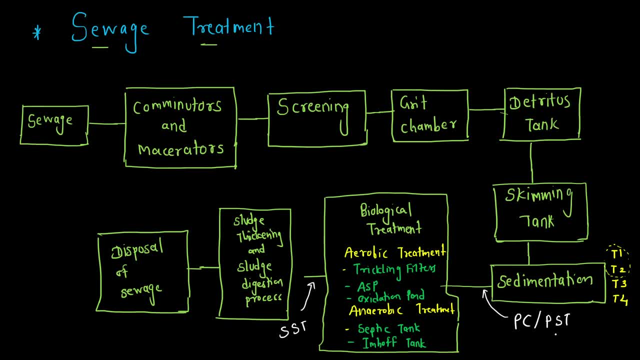 tank. where is the location of this? primary sedimentation tank is located before the biological treatment starts? secondary sedimentation tank is located after the biological treatment is completed. okay, let's say, trickling filter is there. so, after trickling filter, the next step is the tripling filter. now, first step, yoe can use a 됩니다 filter. ok, so 有.